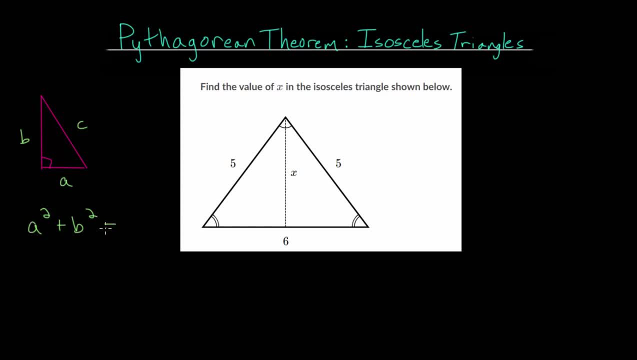 you add them together and you square them each that this is equal to the hypotenuse squared. Remember, the hypotenuse is just the long side of your right triangle and it's always opposite the right angle. So we can use the hypotenuse to find the right angle. So we can use the hypotenuse to 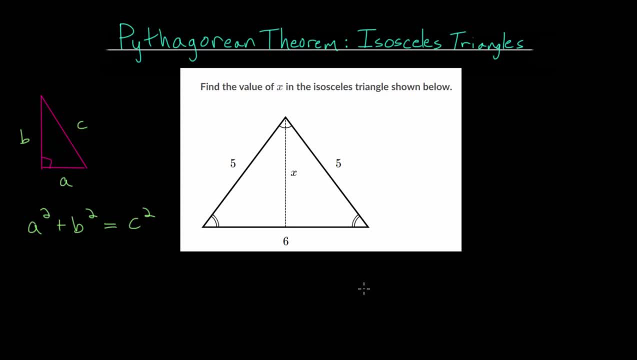 find the right angle. So we can use the hypotenuse to find the right angle. So we can use the Pythagorean Theorem to find one of the missing side lengths. Now, the main idea with this problem is that this vertical line essentially splits the triangle into two congruent right triangles. 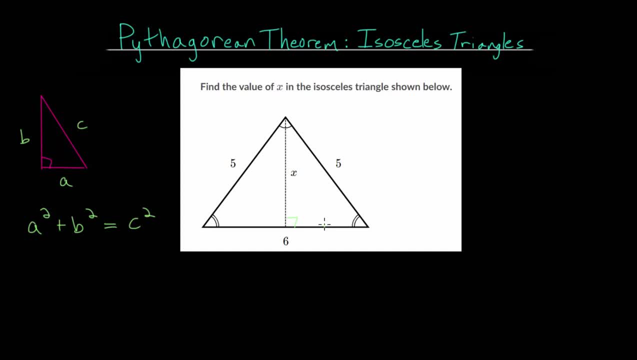 So this is going to split at a right angle and this side length here and this side length here are equal to each other. So you might ask: how would we know that? And that's a little bit complicated, But basically noticing that these two triangles, 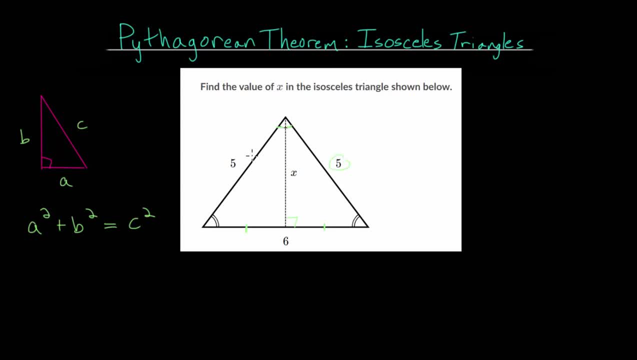 they share one equal angle up here, they share a side length and they share another equal angle down here. So that is the angle side angle congruence between two different triangles. So that would prove that these are two equal to each other, which means that this side length and 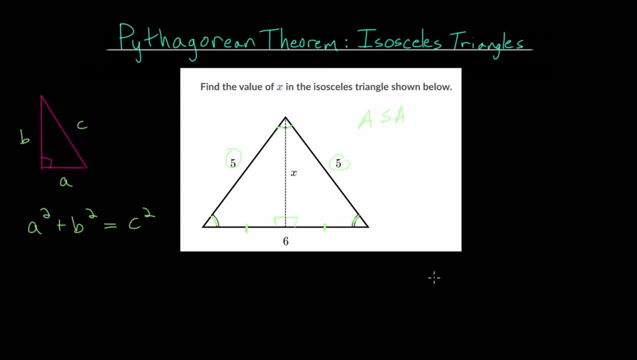 this side length and also these two angles. these must be equal to each other. Okay, We're going to be equal as well. So that's how we would know that those two side lengths on the bottom are equal to each other. but the main idea is, we can use this information. 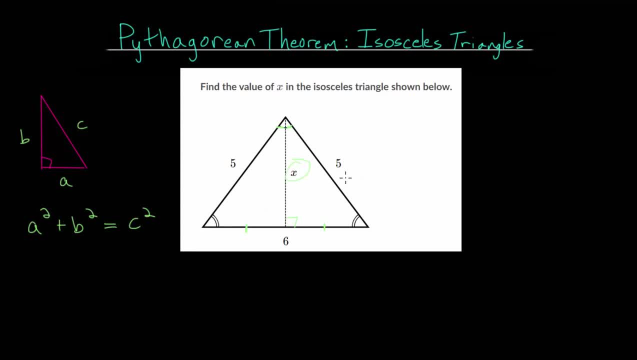 and the Pythagorean theorem to find this missing side length. So, since this bottom side got split into two equal sides, we now know that these are each of length three, And I do also want to mention that we know this is a right angle because we 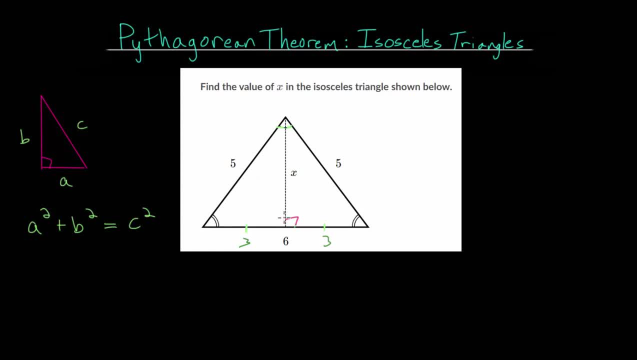 found that, since these are two equal triangles, this angle here and this angle here have to be equal to each other and they're also supplementary, so they have to add up to 180, and if they're both equal, that means they both have to be 90. So we have this right triangle, which means we can use the 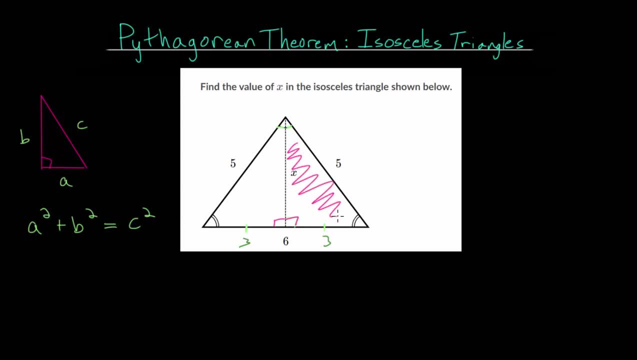 Pythagorean theorem. So let's just focus on one of these triangles and set up our relationship between the side legs. So we can call the legs A and B when matching it up to the theorem, and it doesn't matter which you call which.